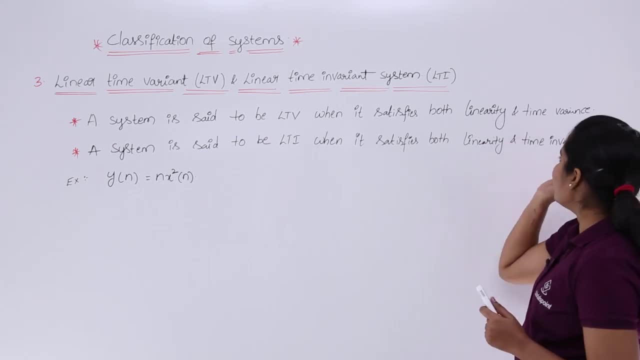 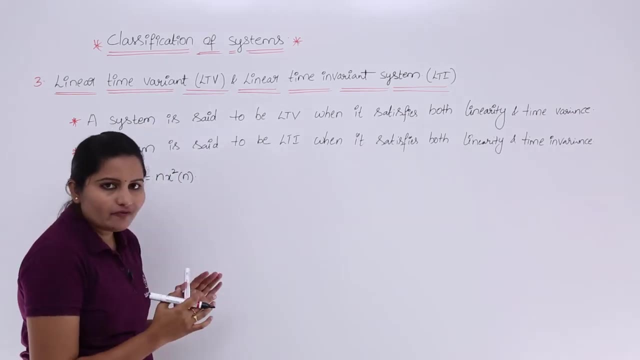 when it satisfies both linearity and time invariance. So, for example, I am considering a problem to explain this. So I am considering a system with a response like this: This is a system response. Now we need to judge whether the system 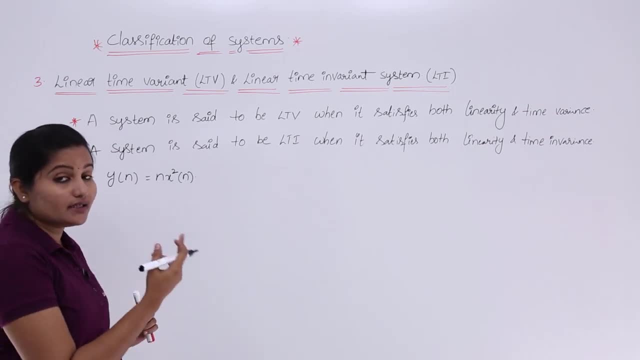 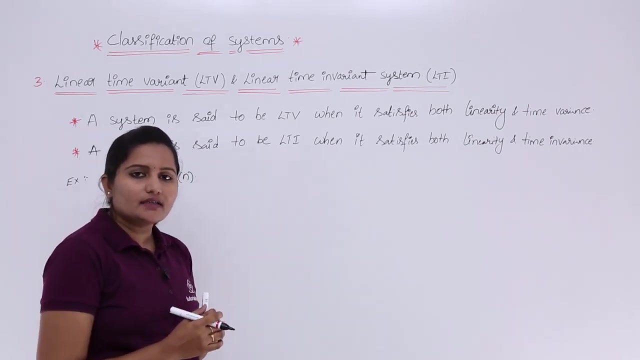 is LTI system or LTV system. that means linear time variant system or linear time invariant system. For that we need to check both linearity and time variance and time invariance. So here to check linearity. so how we can check the linearity means we need to check the. 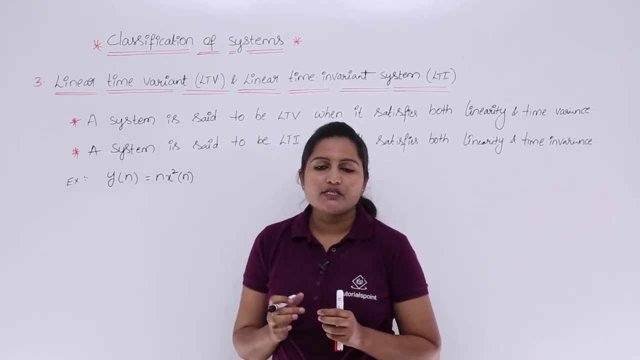 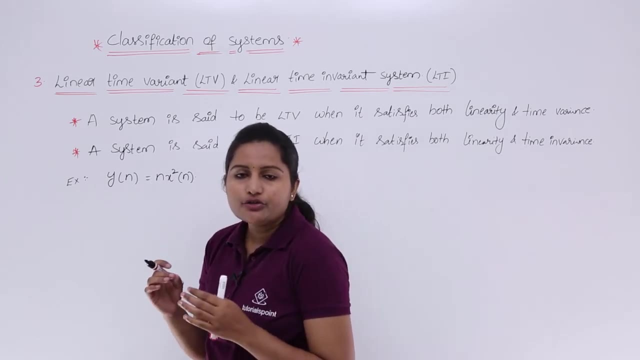 superposition theorem. that means so the individual response must be- is equivalent to overall response. So that means first of all for this system you need to check the superposition theorem. So that means first of all for this system. 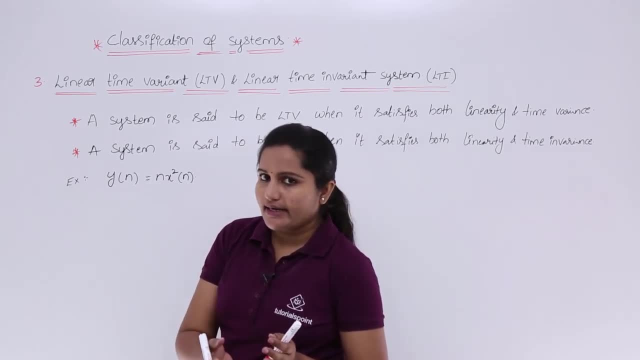 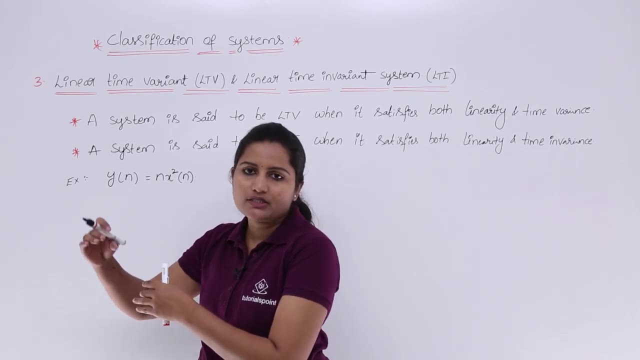 you need to provide a signal, you need to see the response. So second time you need to provide the second signal and you need to check the response and you need to combine those two responses and just you just keep that aside. So after that you just combine. 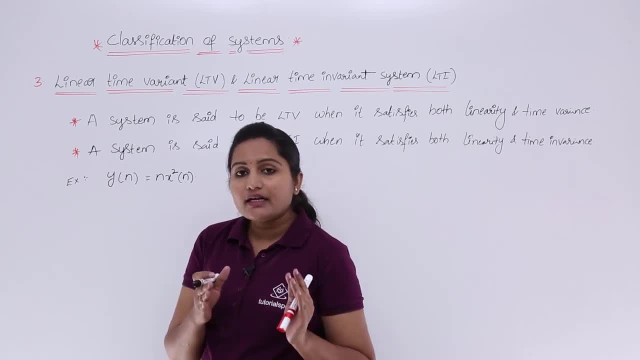 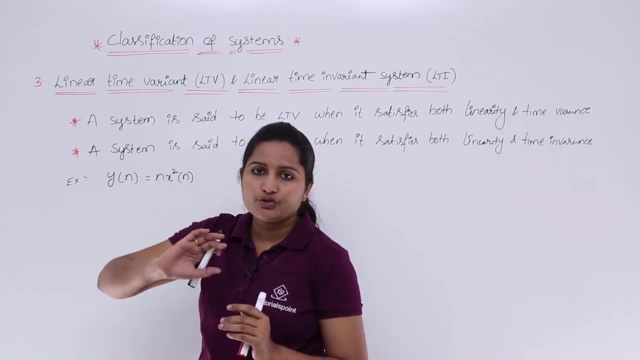 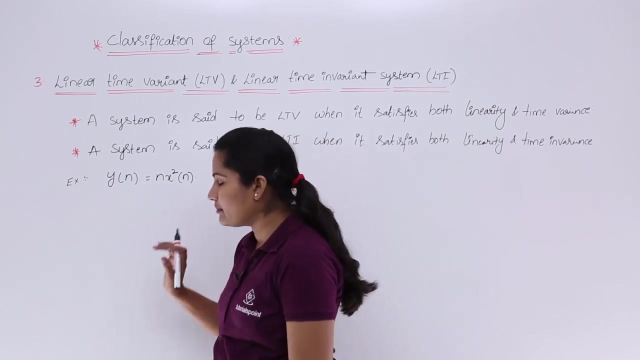 the input signals which you given previously and you can give like a combined signal as input. whatever response you are getting, that response must be equivalent to individual added response. So if that is satisfied, then you can give like a combined signal. So if that is satisfied, then linearity is said to be satisfied Now. 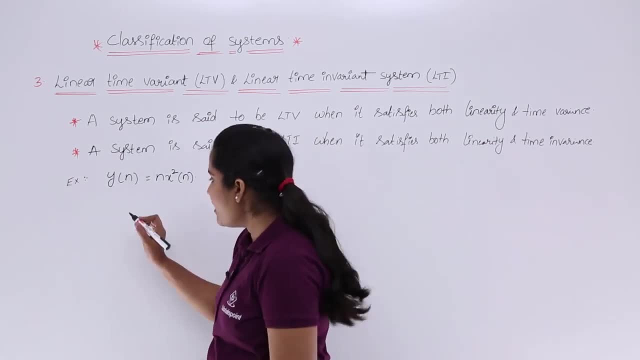 I am doing that. So I am checking for linearity For that. I want to see my y 1 of t. So y 1 of t is equivalent to transform of x 1 of t. that means I am going to transmit my x. 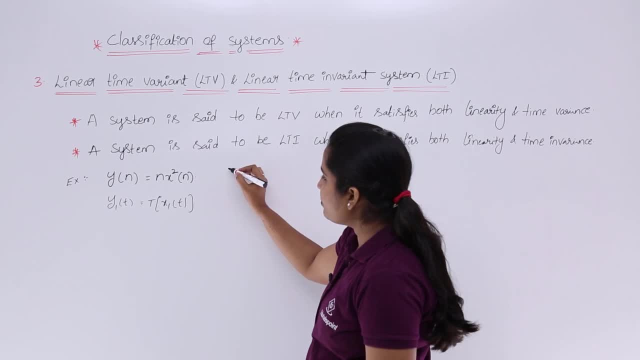 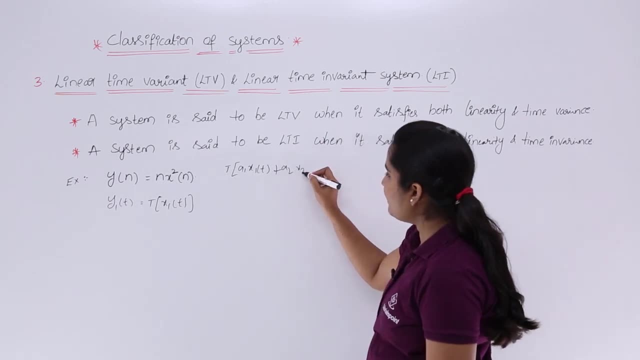 1 of t. So linearity principle is so: transform of a 1 now a 1 x 1 of t plus a 2 x 2 of t, minus a 1 y 1 of t means your x 1 of t plus a 1 y 1 of t. plus a 1 y 1 of t plus a 2 y 2 of t. 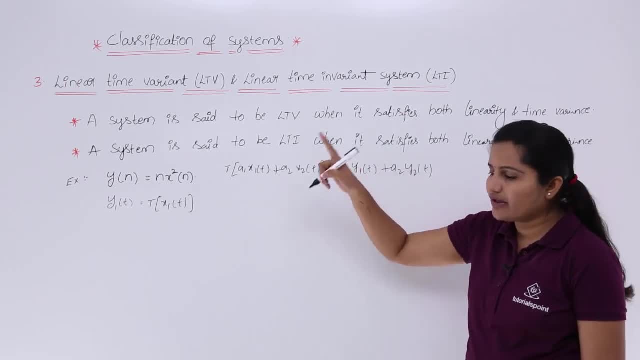 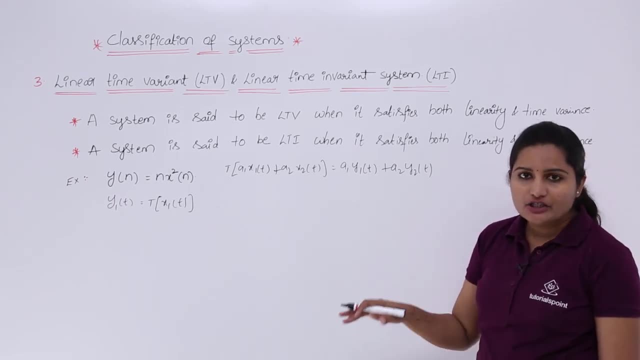 where y 1 of t is the response or output when we give an x 1 of t signal. So where y 2 of t is output of the system where we give an x 2 of t signal. So now so the individual response addition. 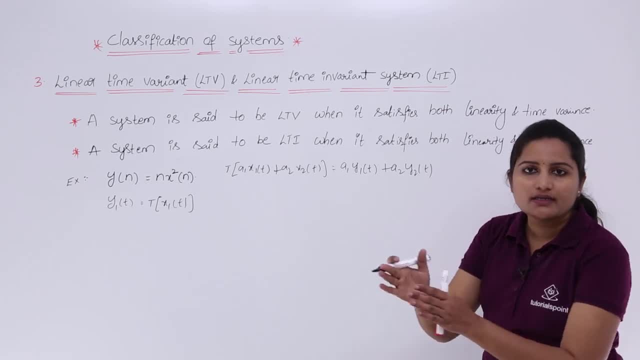 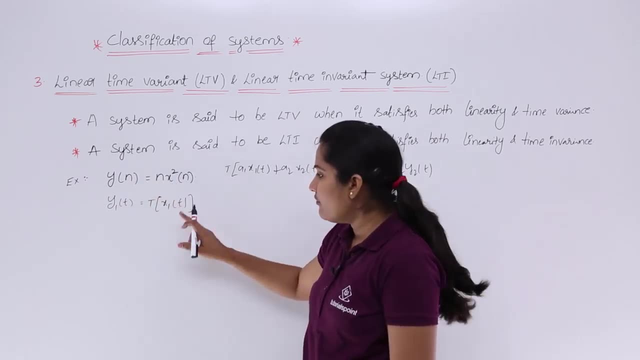 must be equivalent to combine input signals transform. So now I am considering y 1 of t. That means will get y 1 of t. in this system, whenever we transmitted x 1 of t, then the response y of n is said to be y 1 of n. So now, when we are transforming any signal according to the given 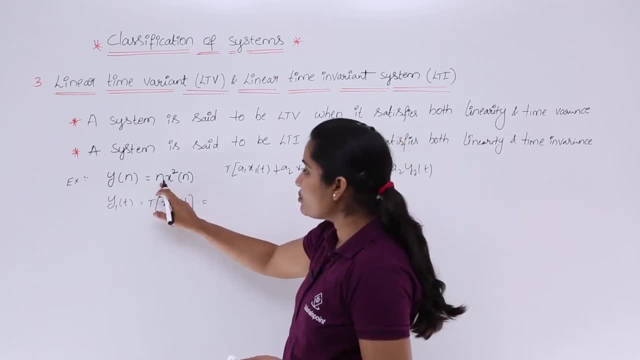 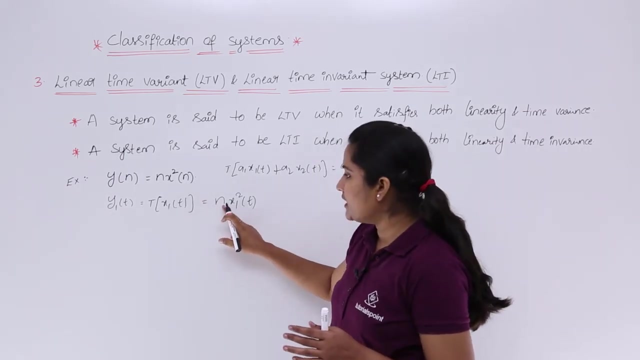 response what the system is doing. it is going to multiply with n. So n into x, 1 square of t will come. that means so whatever system is doing means it is multiplying with factor n and it is squaring. So whatever signal we are giving, for that signal we need to multiply n and we need to. 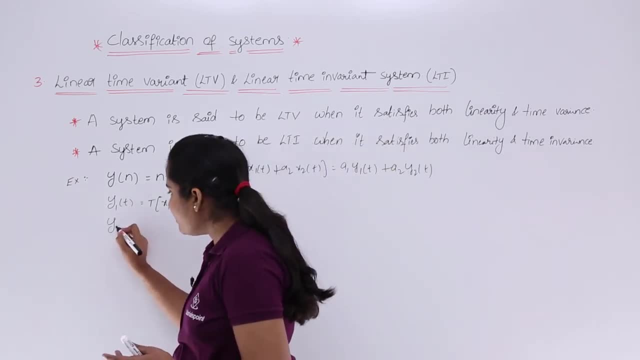 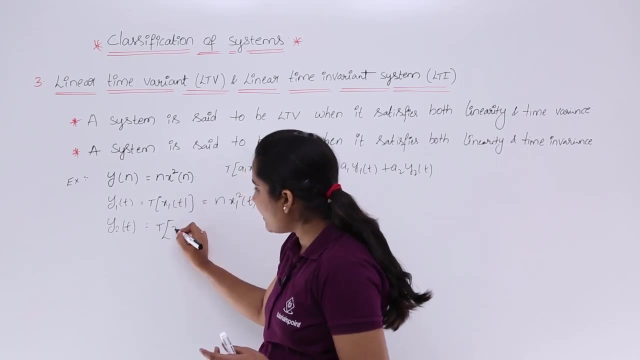 square that signal. Second time I want to give x 2 signal. So by that I used to get y 2 of t as my response. So that means this time I want to transmit x 2 of t to through that the same system. 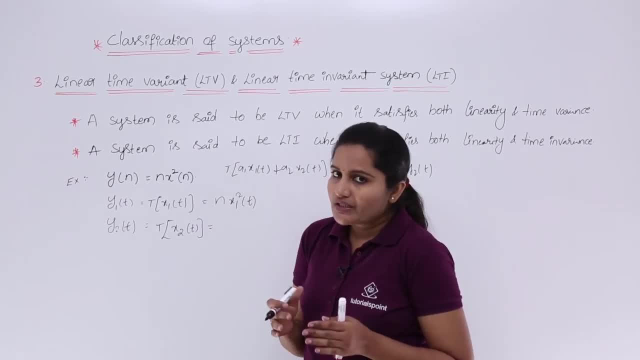 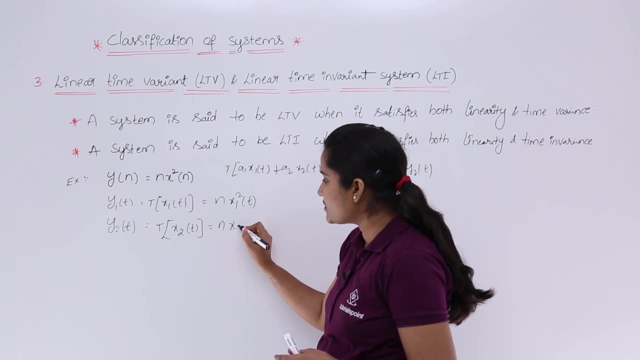 So same system, so system. do not want which signal is coming, it just do its process. that means it is going to multiply the given signal With n and it is going to square that signal. So the response this time is equivalent to x- n. 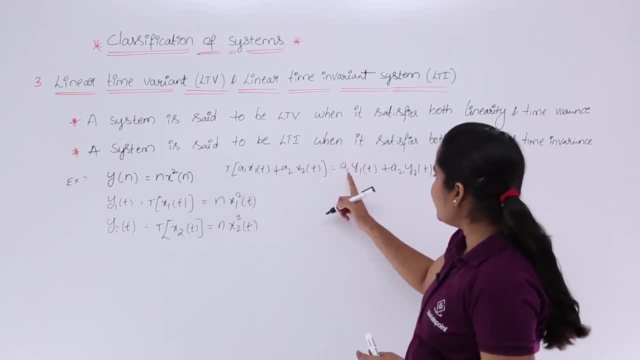 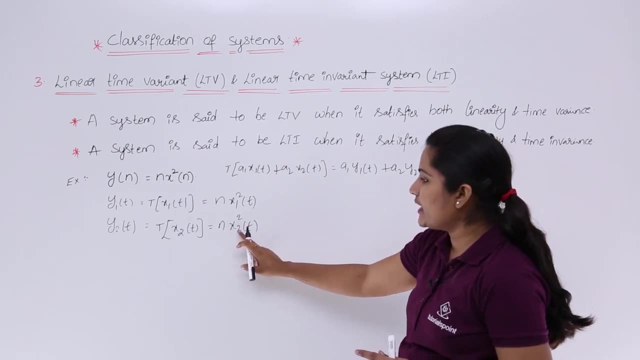 into x 2 square of t if you substituted in this. So you are going to get, ah, some equation like a 1 n x 1 square of t plus a 2 n x 2 square of t. like that you are going to get. So now we are. 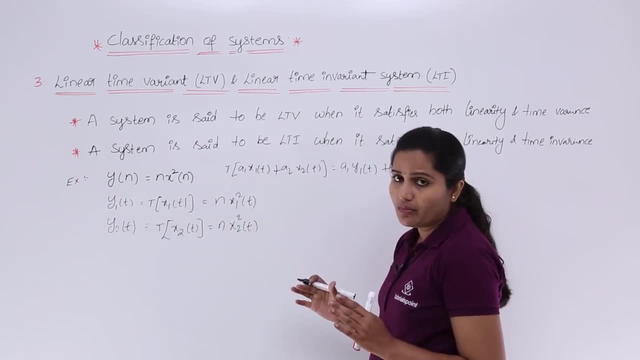 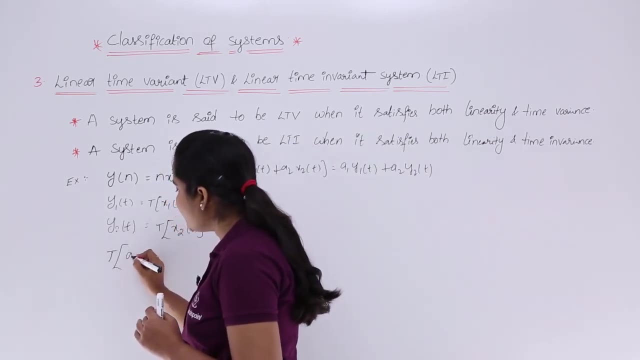 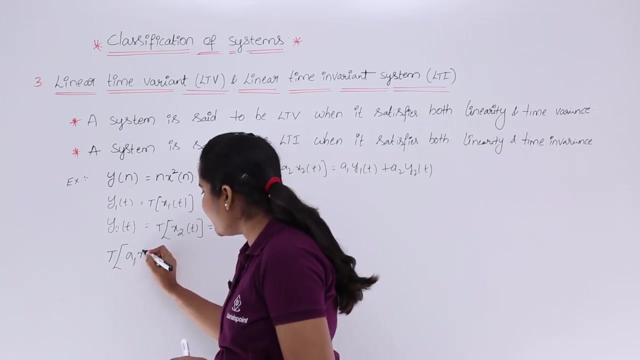 going to calculate the total transform or total combined response of the system. If you transform the combined signal, that means at the in input itself. if you are combining not the responses, So at the input itself, you are combining your signals, which are previously given, and you are 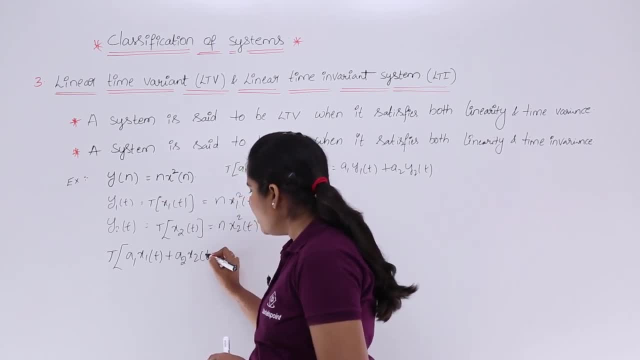 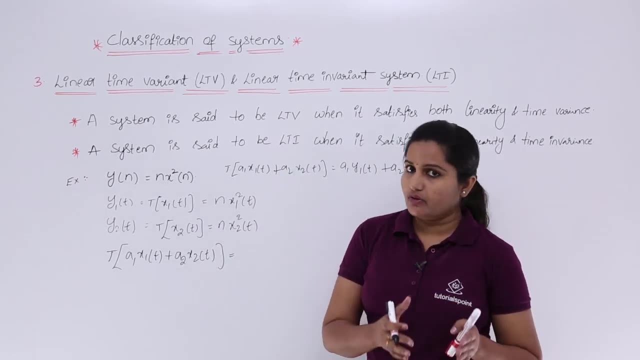 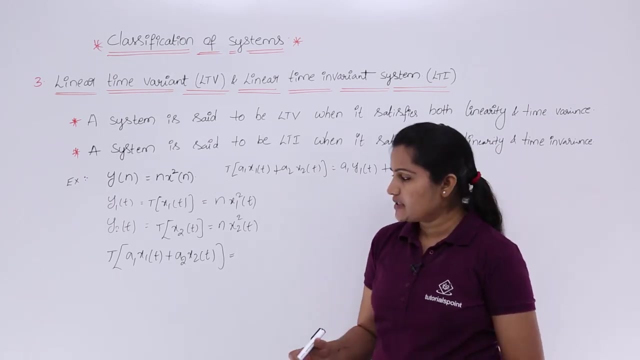 you are giving like a new signal, then what you are going to get Here- also system do not see whatever. whatever we are giving, that is, that may be a combined signal, that may be individual signal. We are giving for that signal. ah, whatever we are giving for that system, that system is going to. 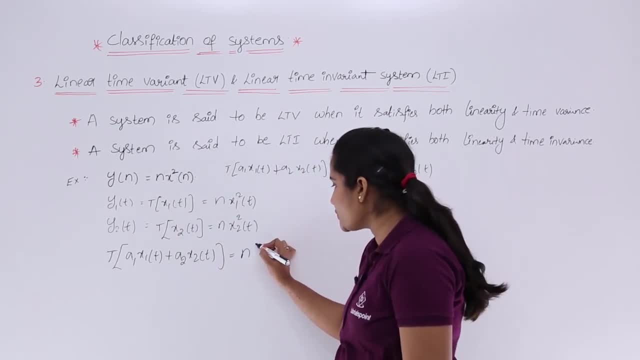 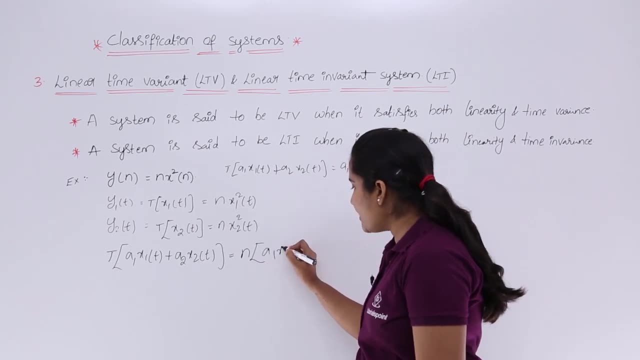 multiply the given signal with n and it is going to square. that means n into the signal given is that means in place of x of n. So we are providing x, 1 of t plus a 2, x 2 of t, whole square. 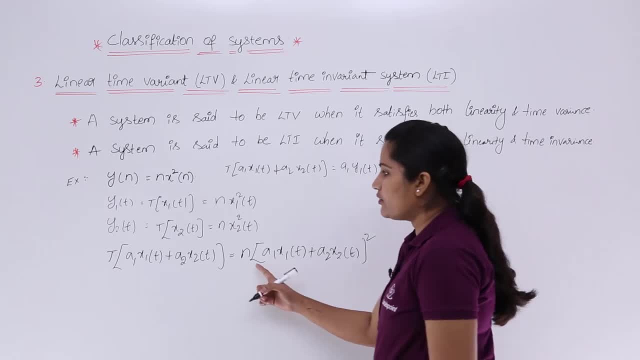 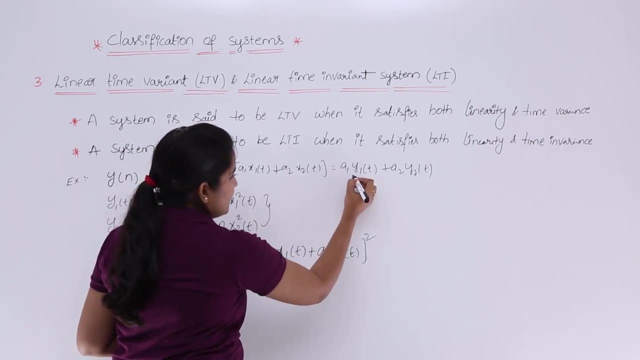 So whole square like this we are going to consider. So now you can imagine. So if you, if you consider this path, if you consider this path, then it will be a 1 into y. 1 of t mean n? n x 1 square of t, plus a 2 into y. 2 of t means n x 2 square of t. 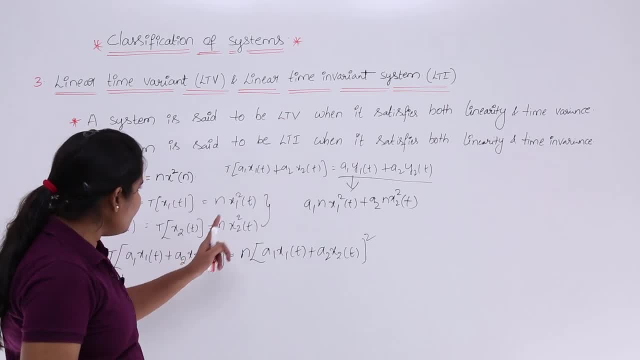 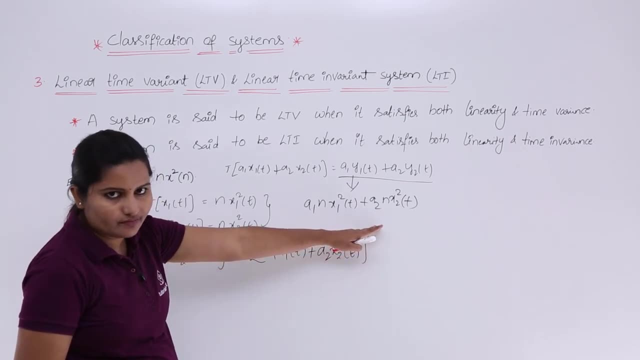 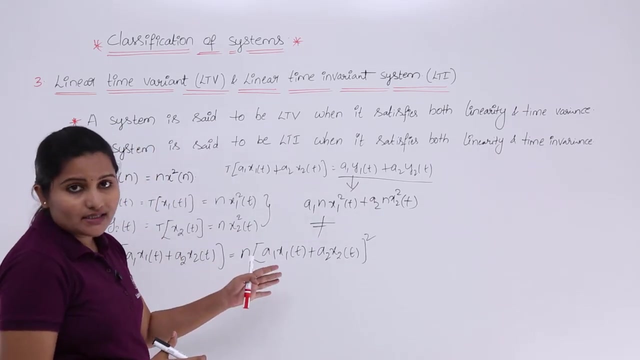 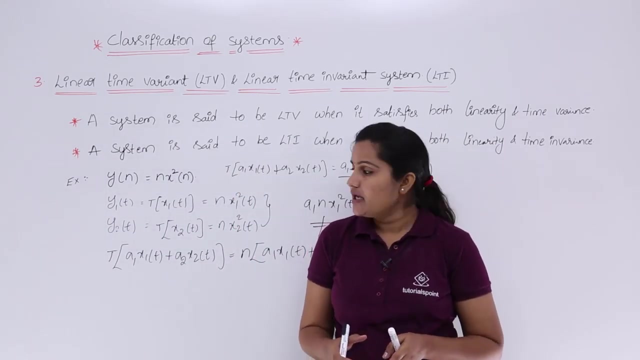 So this is this value. but here, when you transform to the combined signal, if you see this equation, this cannot be equal to this equation. So this is not equal to this equation. So we can say: So this is a non-linear system. as I told you in the, in the checking of linearity and non-linearity, that means linear and non-linear system. as an example, ah, I considered some x square of n or x square of t, something like that. 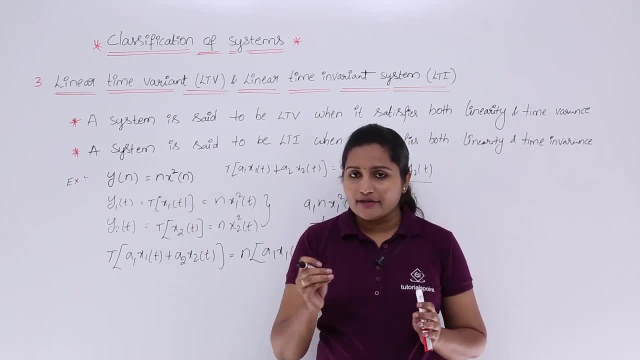 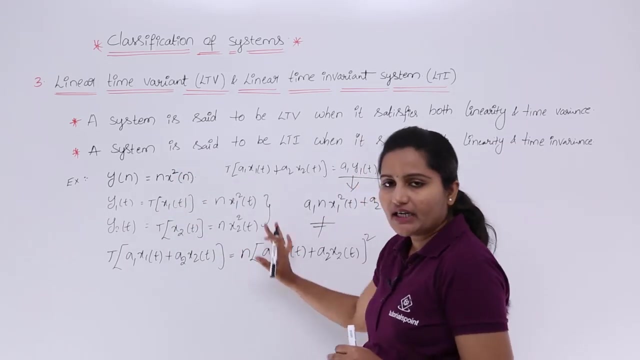 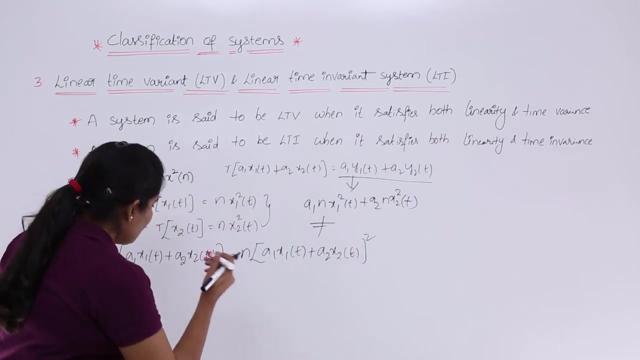 So there also. so whatever I told you that ah, as it simple trick for technical exams, whatever signals we are having squares like that, So the those are not said to be linear, that means non-linear. So here, So here also, we consider square means. so definitely, without this searching or without this checking, you can say this is non-linear system. ok, this system is non-linear. 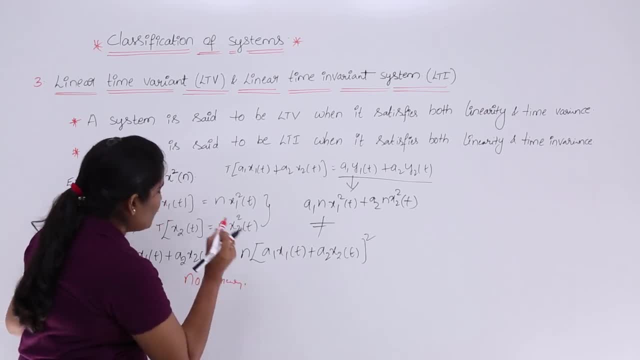 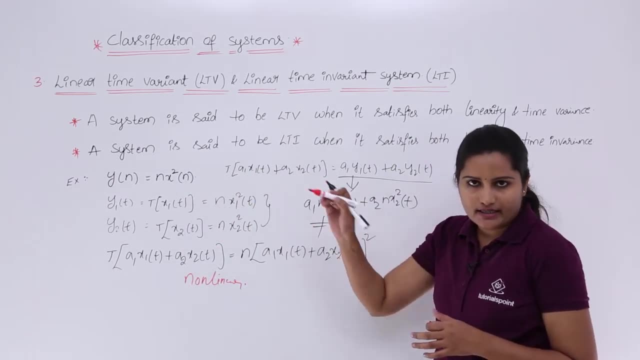 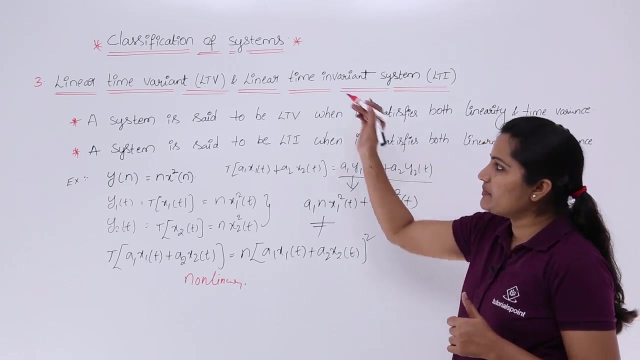 So we searched for linearity. so this system. so, ah, this system is said to be non-linear by this response. So now we need to check for time variant and time invariant to justify whether the system is LTI or LTV. So now, 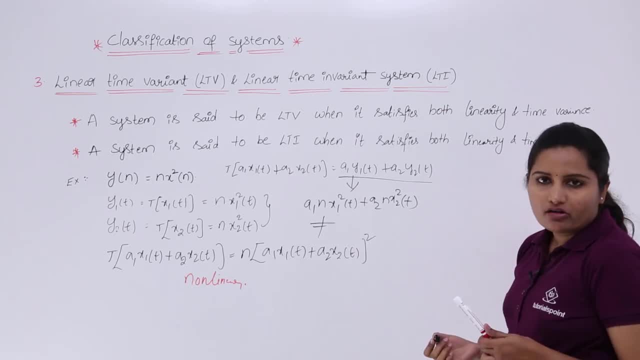 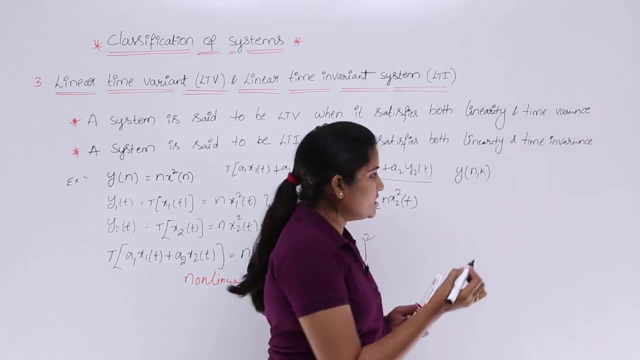 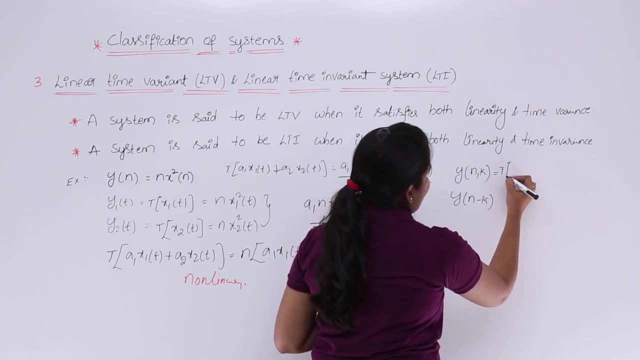 So now I want to check so time variant or time invariant? for that I need to consider y of n comma k and y of n minus k. y of n minus k, what is meant by y of n comma k means this is nothing but transform of x of n minus k. 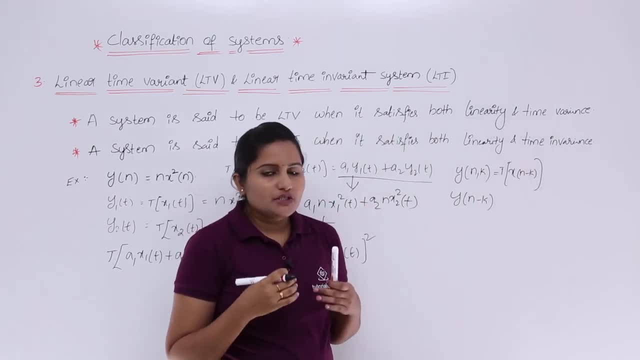 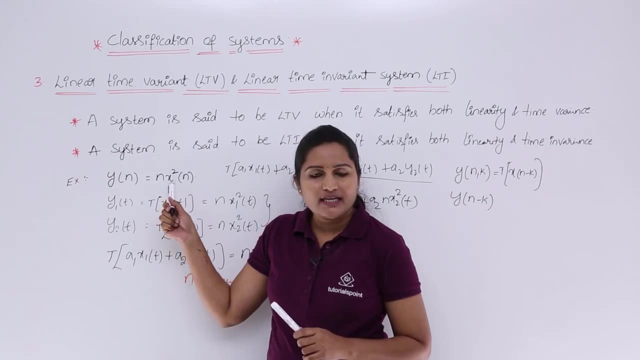 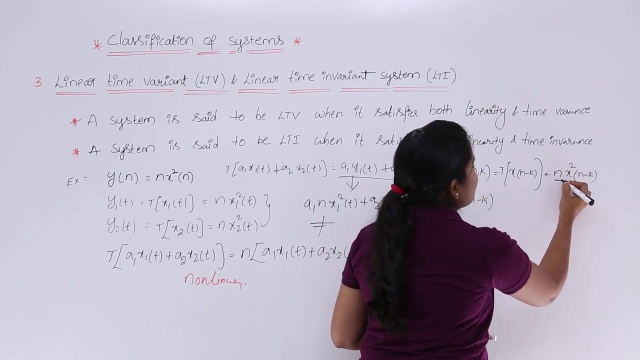 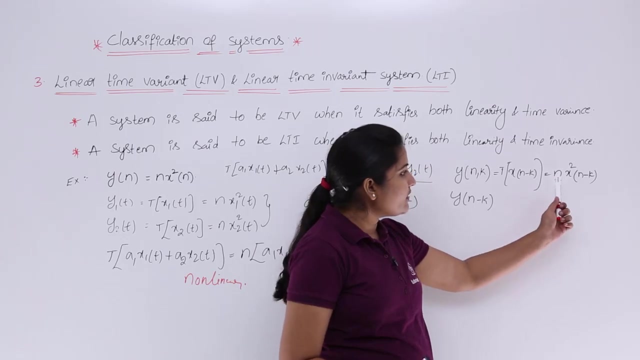 So that is nothing but ah, just delaying the input response by k samples. so whatever input is there that we need to Delay by k samples? so here the input is n into x square of n. the delayed version of this is nothing but. so n into x square of n minus k. we are not going to change the multiplication factor, we are just want to delay the signal. so that is why only in the signal we delayed. so whatever n here we are having, there we are not going to change anything. the multiplication factor will remain as it is. 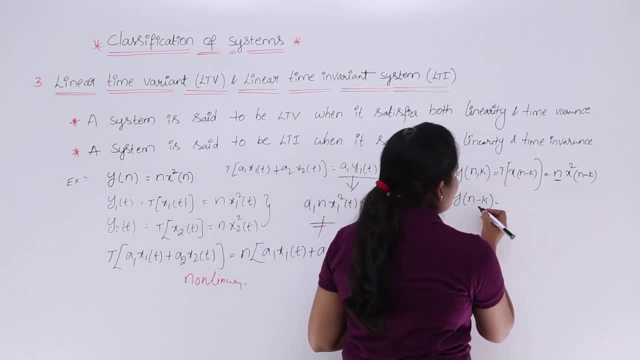 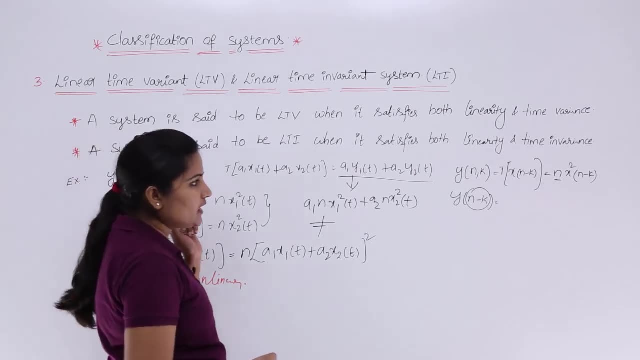 So now coming to y of n Minus k, here this is nothing but just substituting n minus k in place of n in this response. so here you can change this n why? because we are not delaying the signal, we are just substituting the value for n. 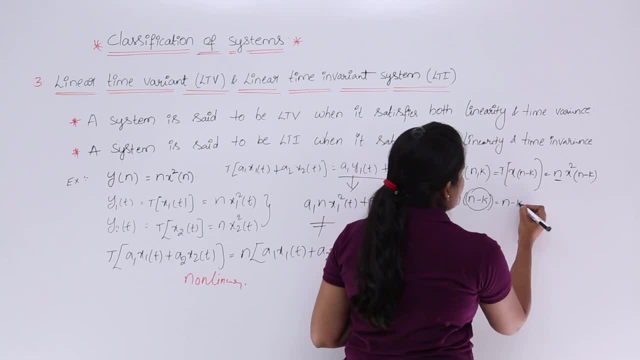 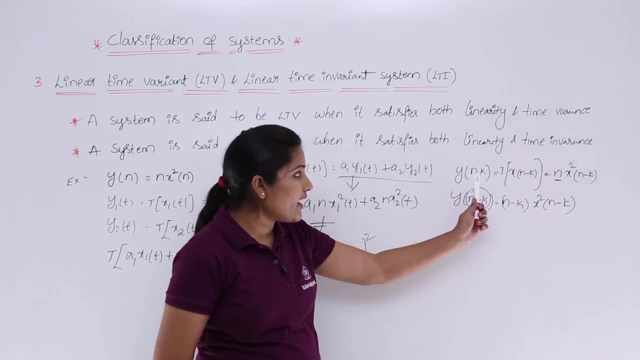 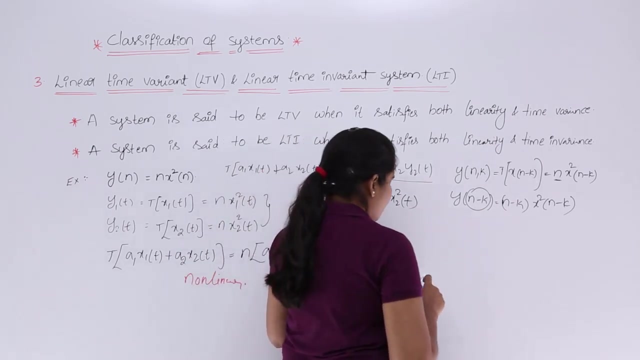 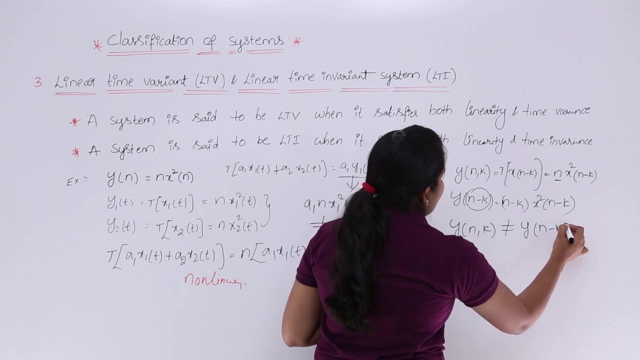 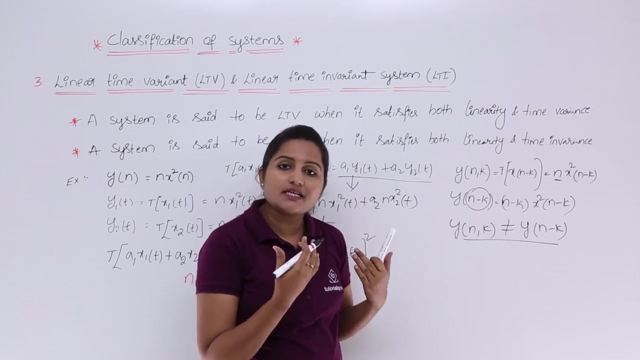 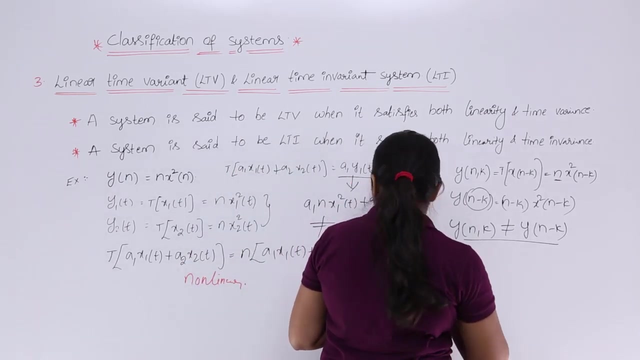 So that is why you can change this n n minus k into so x square of n minus k. so if you observe the values of y of n? n comma k and y of n minus k, So these You are not said to be equal. that means so y of n comma k is not equal to y of n minus k. so by this you can say your input change is not equal to output change. so system is varied. that means time. system is varying with time. so you can say this is time variant system, this is time. 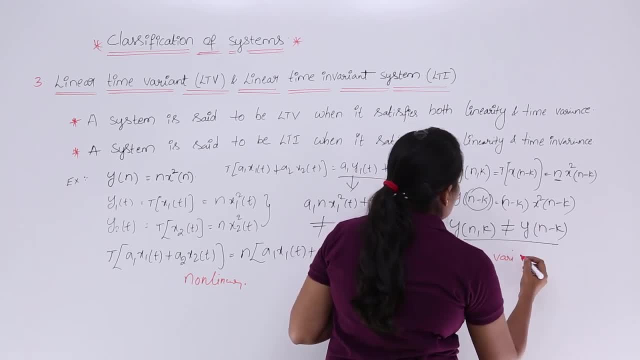 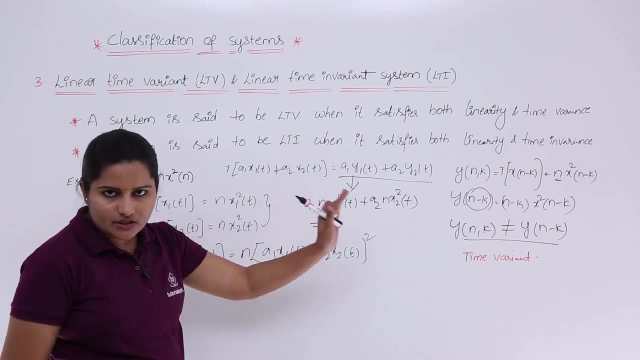 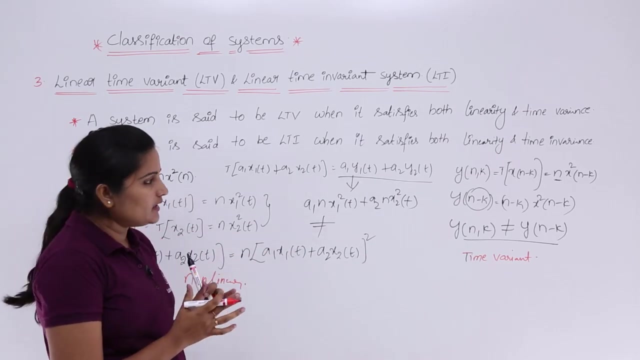 Variant, Variant system. so here, if you observe these two, if you observe these two, then you are going to get: so this is non-linear and this is time variant. so definitely this is not at all LTI and not at all LTV. why? because a system is said to be LTI or LTV, it must satisfy linearity, so no need to search for time variance. also, here itself, you can say: this is: 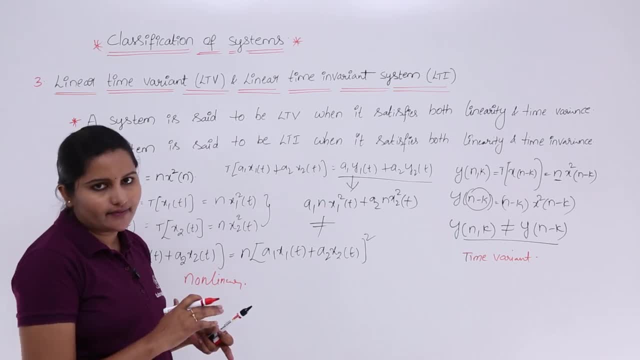 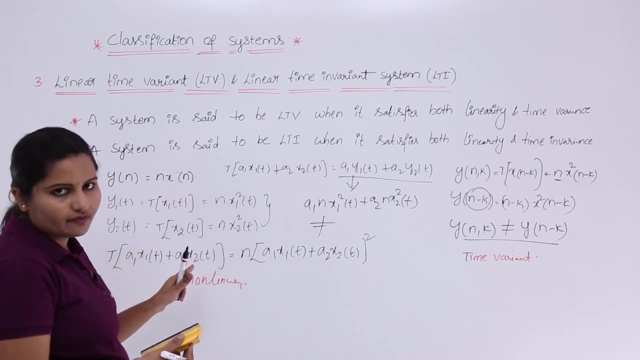 A, Not at all. LTI, neither LTI nor LTV. for example, if a system is given like this, for example, a system is given like this, without square, if they given, then how we can do here, we are not having any square. when you calculated y1 of t and when you are calculating y2 of t, you are going to get just n into x2 of t. 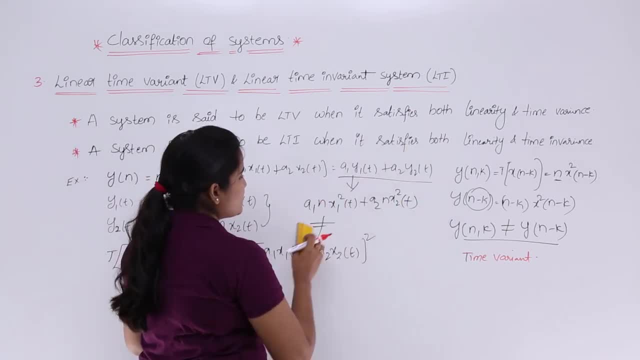 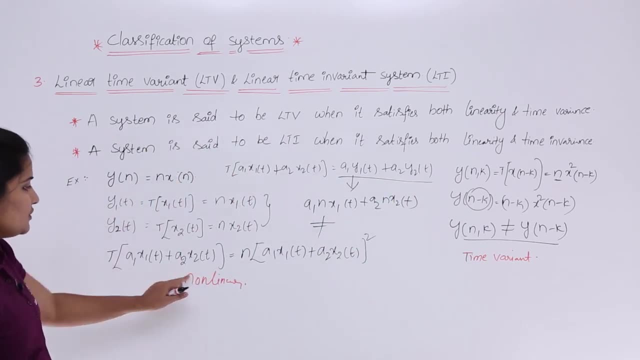 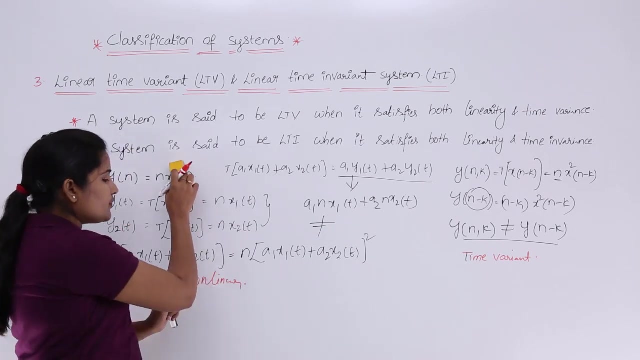 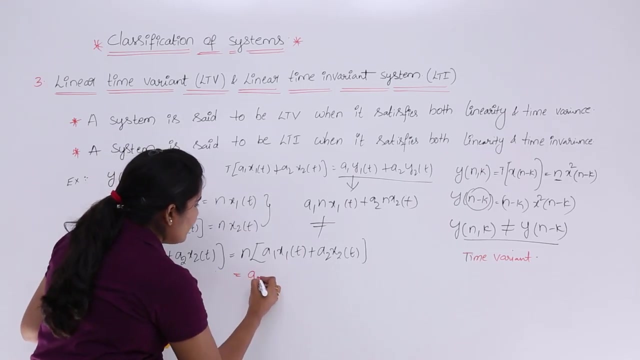 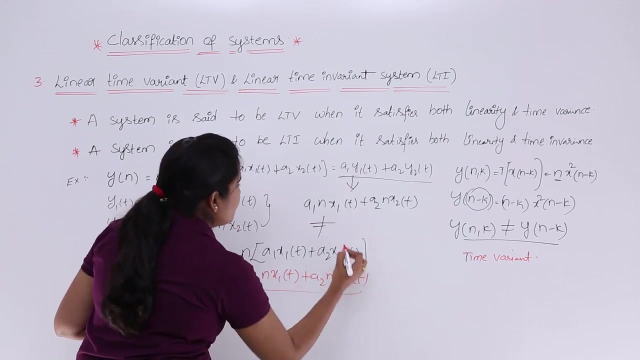 So here, if you combine these two responses like this, you do not have square here. So you Simply you are getting like this. so when you consider the total response, that means combined signal, when you given then a1, x1 of t plus a2, x2 of t, as we are not having square here, you are not getting square here, then here this is equivalent to a1, n, x1 of t plus a2, n, x2 of t. if you see these two now, these two are equal, so you can say linearity principle. 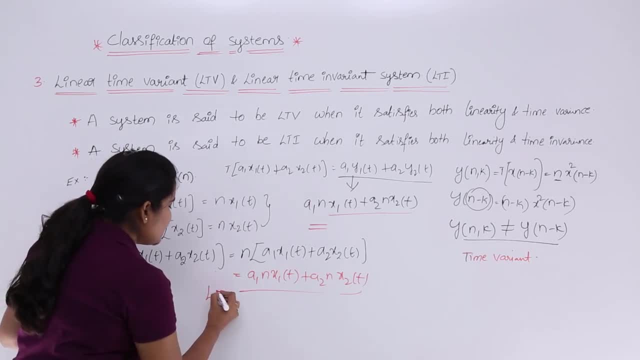 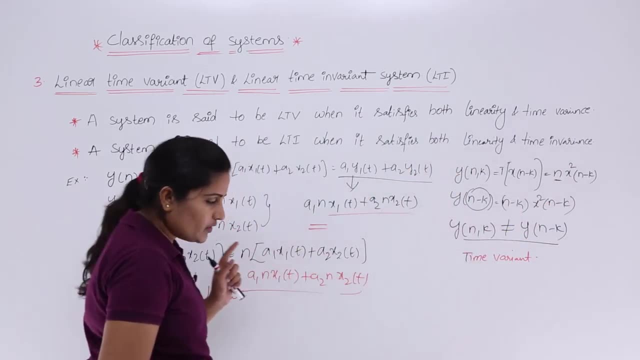 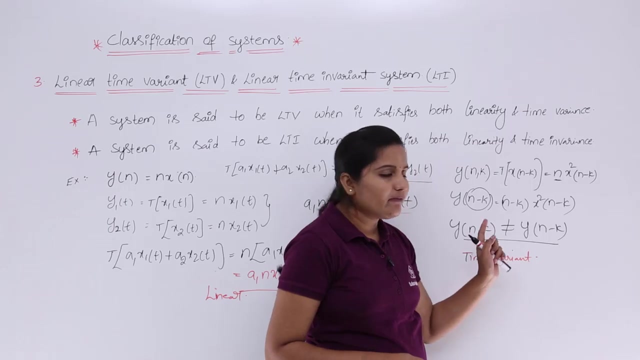 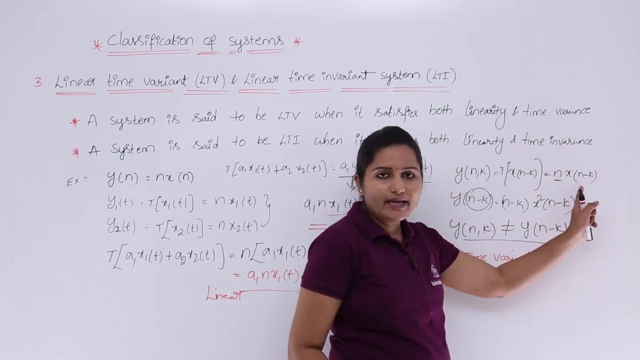 Is obeyed. so that means so this system is linear. this system is linear. now now coming to here what we need to change. so now we consider a different system. so n into x of n. you need in that also to calculate time variant or time invariant. you need to delay your input by k samples. you need to delay k by n. k samples means n into x of n minus k. only in signal you are going to get 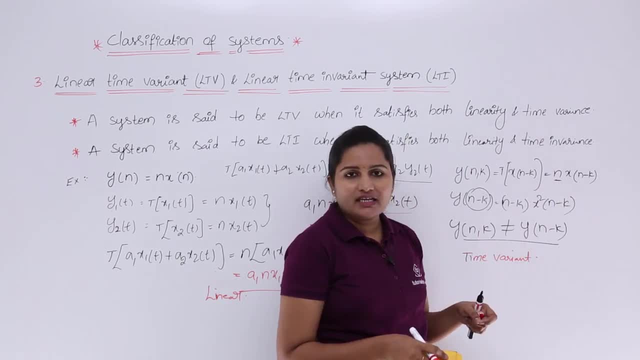 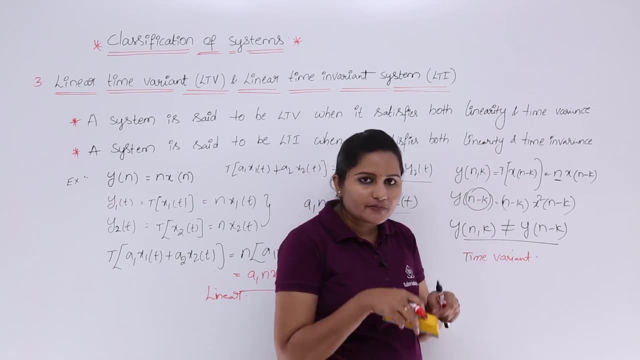 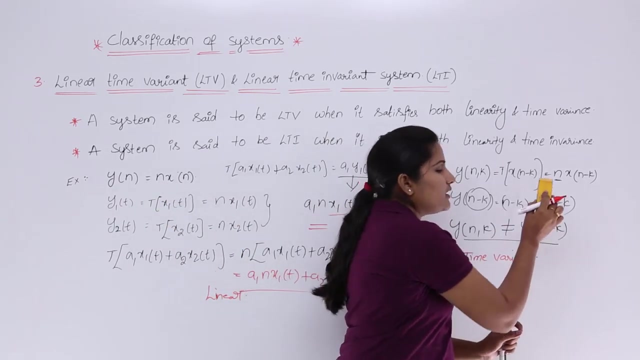 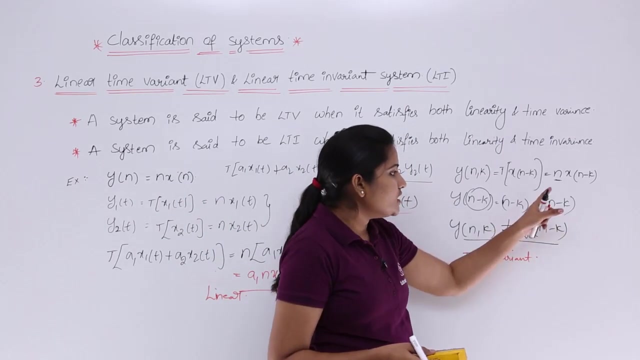 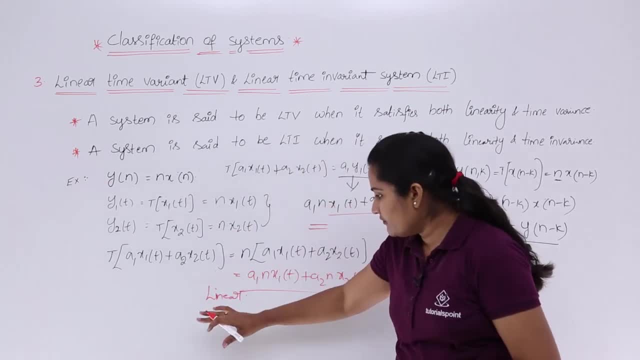 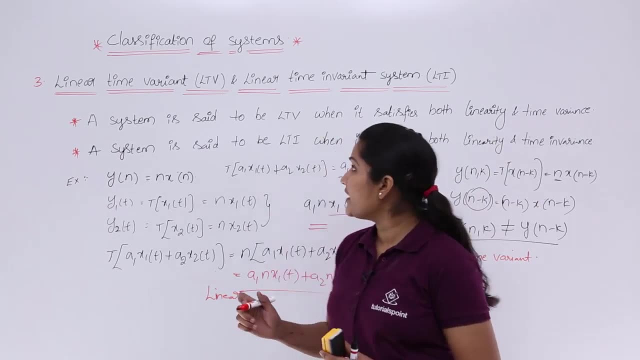 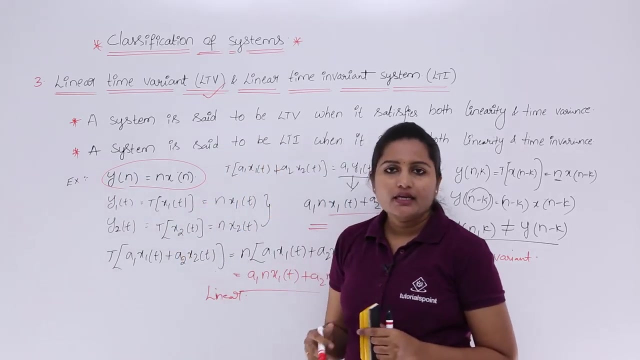 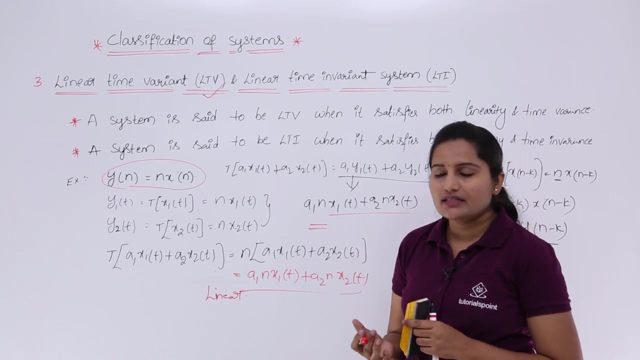 A. So if this is time variant, then if this is linear, you can say that is linear time variant system. linear time variant system is LTV system, So a system with this response is said to be linear time variant system. For example, if you are having any other system like this, 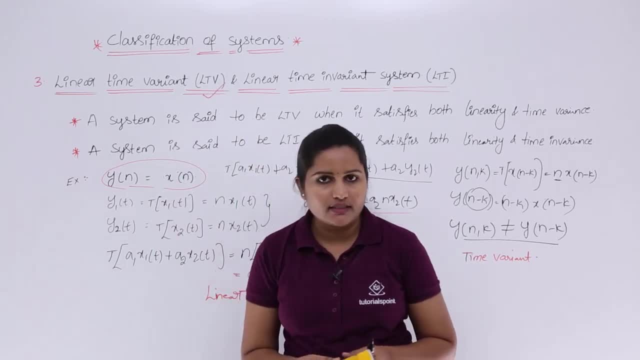 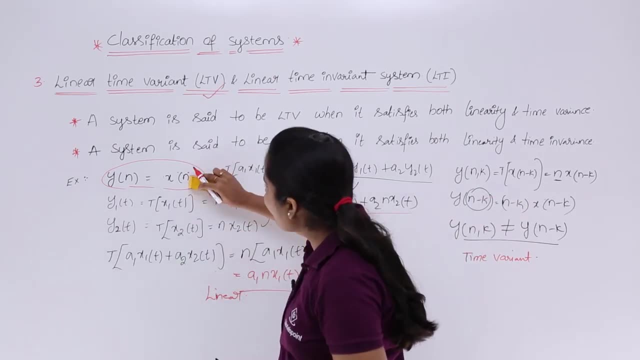 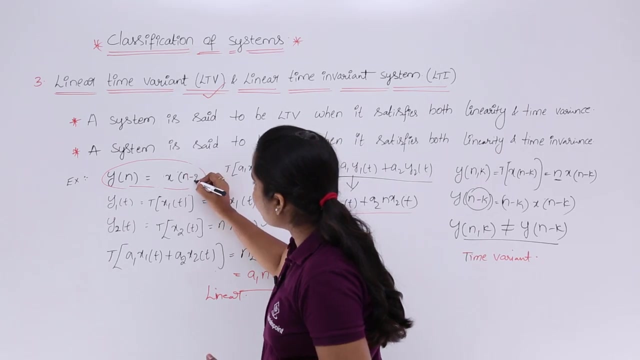 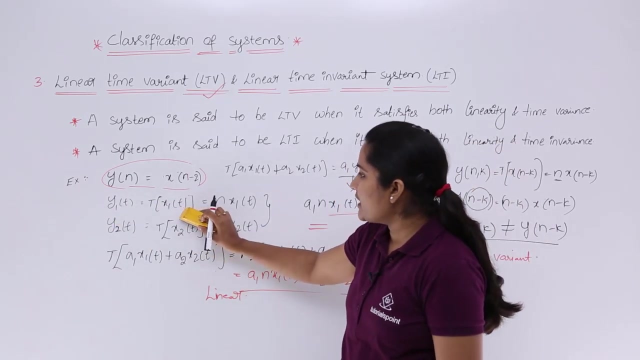 so x, x of n, like this. if you are having x of n like this, then how you are going to calculate x of n or x of n minus 2? you can say So, for example. I will. I will consider another one. another example: if you are having x of n minus 2, definitely y 1 of t equal to x 1 of t. So 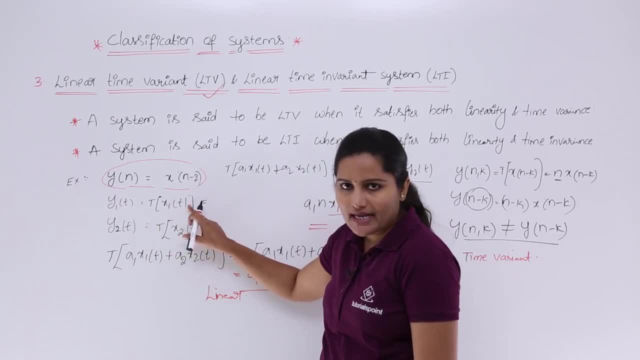 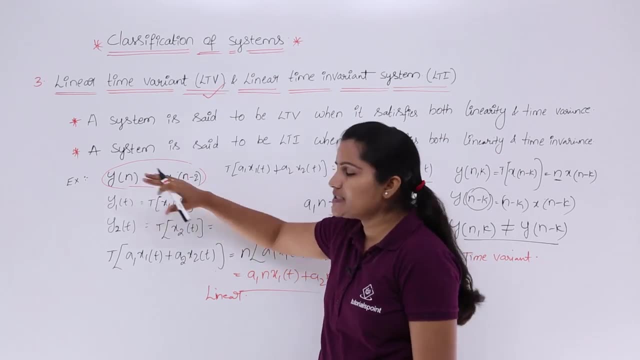 here y 1 of t equal to transform of x 1 of t. when y 1 of t will come, whenever we are transforming x 1 of t through a system with this response, then whatever signal we are transmitting, for that signal. so you need to consider n minus 2. 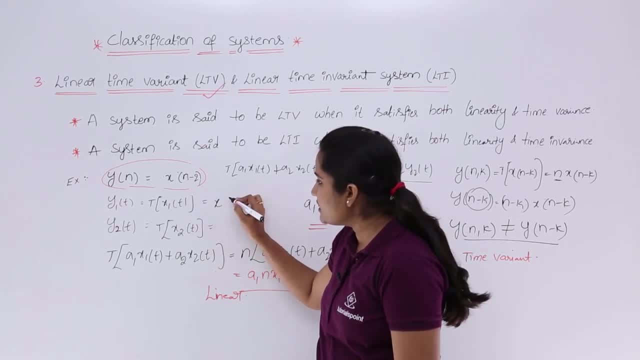 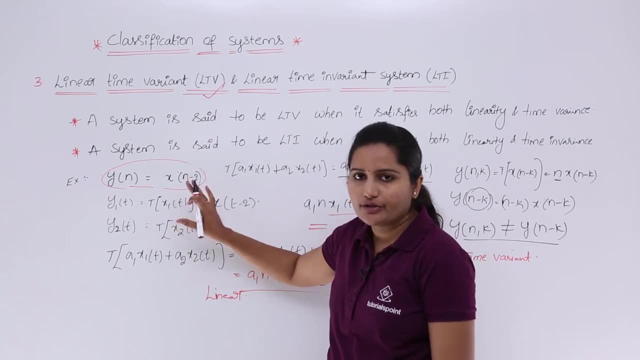 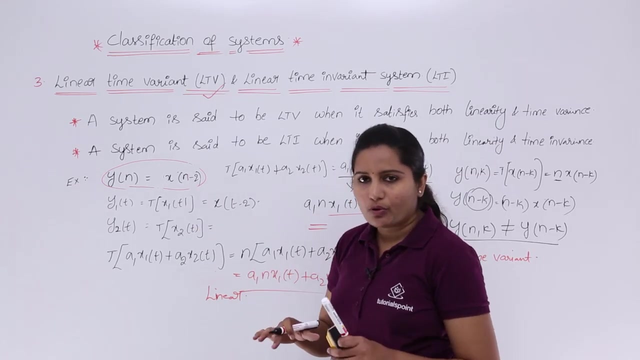 or t minus 2. so here i i need to consider x of t minus 2. don't confuse: here, ah, i consider continuous time, but here in this description i given a discreet time and here i consider continuous time, no problem at all. so here, just for searching, i am considering: so here y 2 of t equal to x 2. 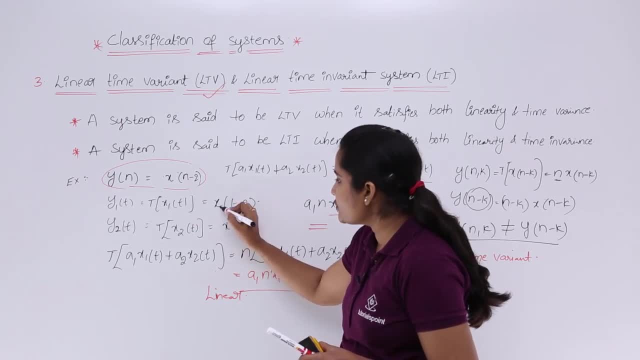 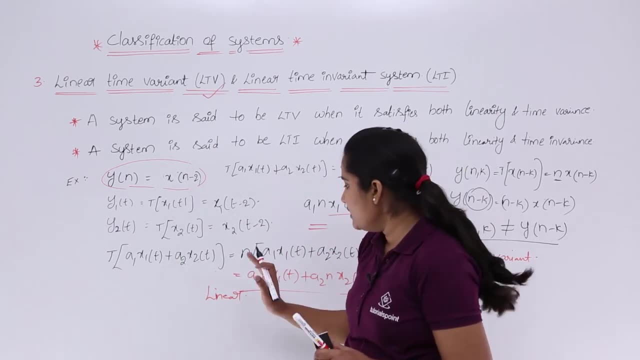 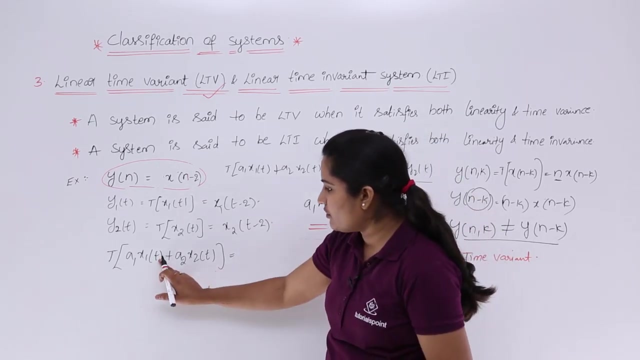 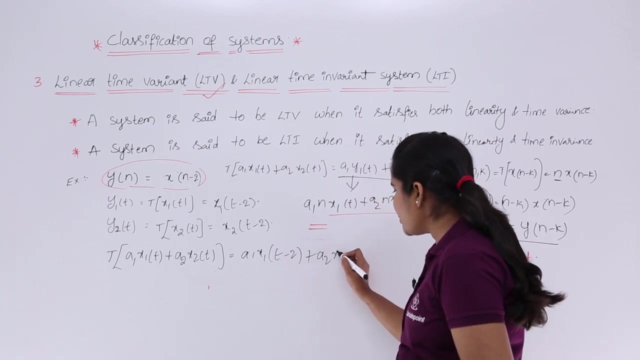 of t, when you are transmitting x 2 of t, so you are going to get x, 2 of t minus 2 again. so now when you are giving combined signal, so here also you are going to get. so like this: that means in each end, every signal you are going to delay by 2, that means x1 of t minus 2 and plus a2 into x2 of. 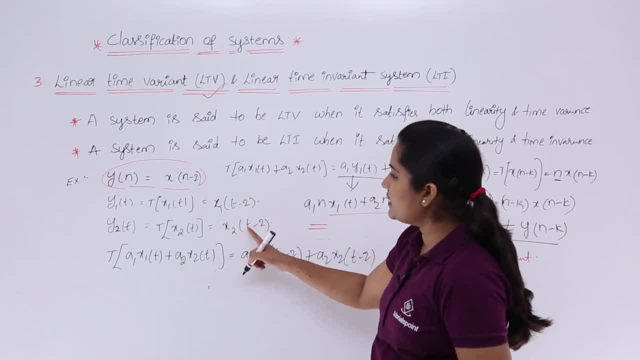 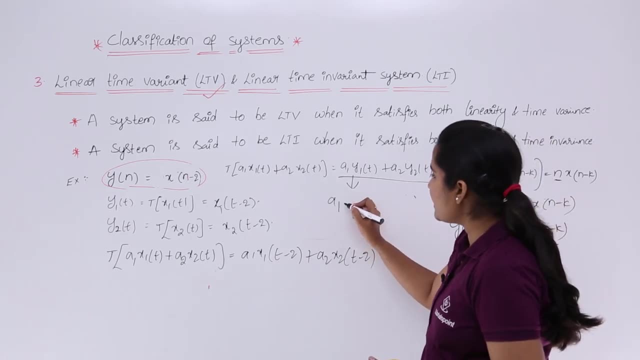 t minus 2 you are going to get. So now, if you can see these two, y1 of t and y2 of t, if you substituted in this, then what you are going to get is a1 into y1 of t is nothing but. 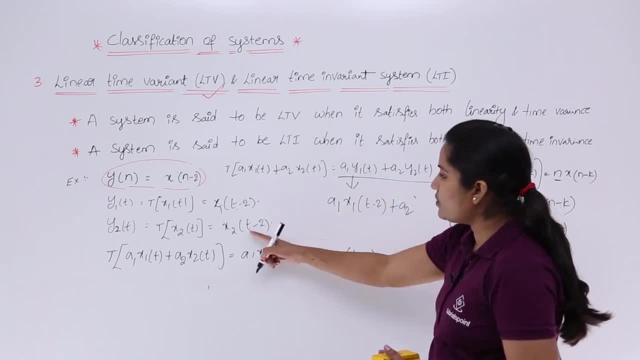 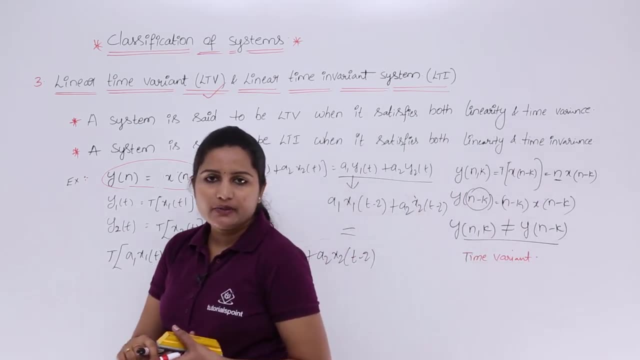 x1 of t minus 2 plus a2 into y2 of t is nothing but x2 of t minus 2.. So these two are equal. So superposition principle and linearity is satisfied, then this is said to be linear system. 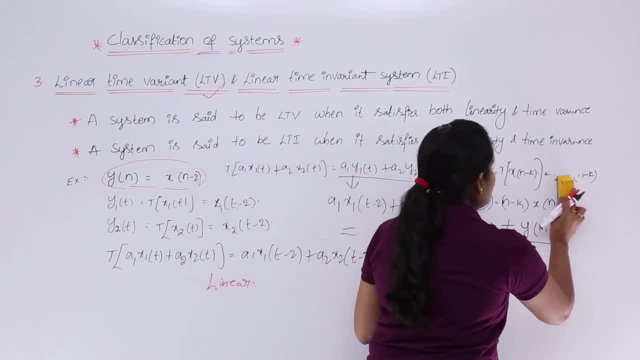 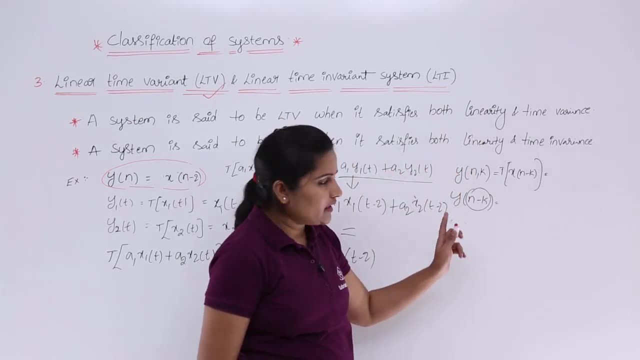 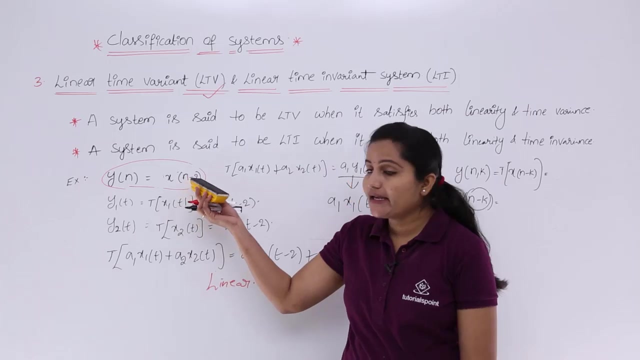 Now coming to here. so here we need to change this, here we need to change this. So here for time invariant and time invariant. so we need to check for y of n minus k. this is nothing but input change. that means we need to delay our signal by k sample. So actually that is x of. 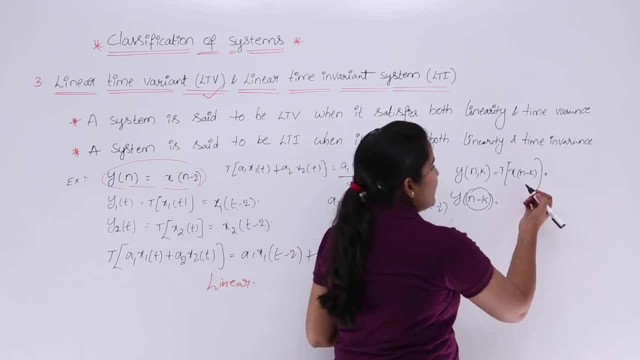 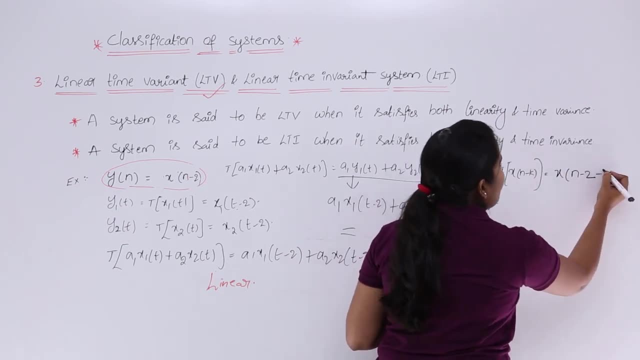 n minus 2 or t minus 2.. So here we need to delay means so again. so x of n minus 2 already is there again we need to delay another k samples, and then here we need to calculate y of n minus k. this is the.